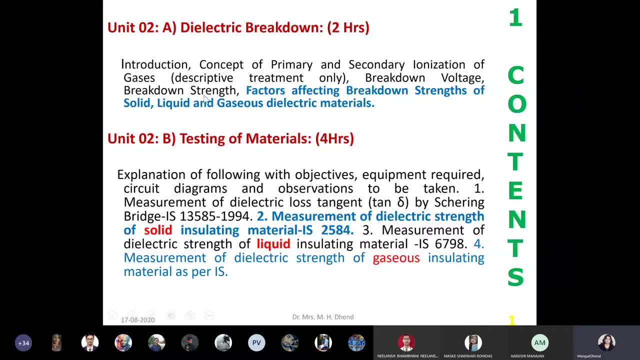 will discuss these two definitions when we will learn testing. I will start with testing first and then we will see this descriptive theories again. Okay, so Unit 2B is testing of material. four lectures are there, So in that four tests are there, you should be able. 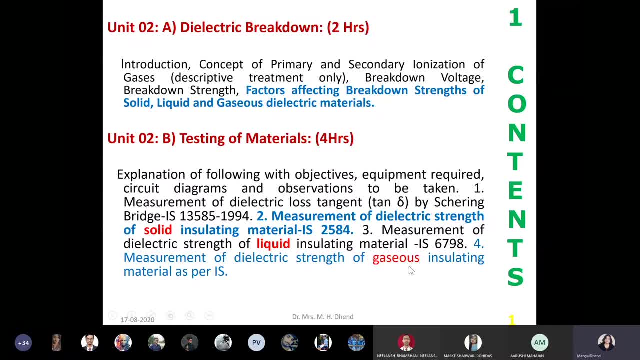 to find out dielectric strength of air liquid solid and loss tangent tan delta. With the help of this, you will be able to find out the strength of air liquid solid and loss tangent tan delta. So we have studied the characteristics, we studied the properties, application, so that 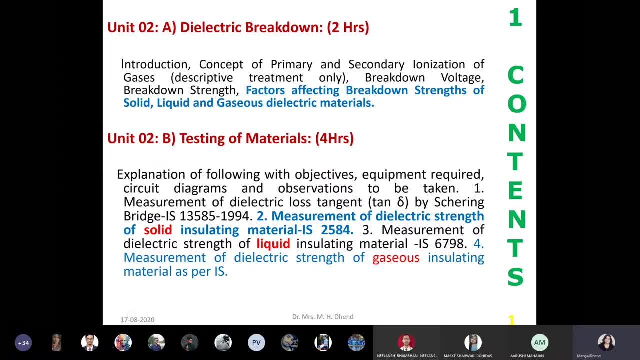 way now to learn. testing is a good sequence of the unit. Okay, so first we covered third unit, so you are in stage. What are the difference? and just now you are written in the test. also, what is the difference between solid liquid? 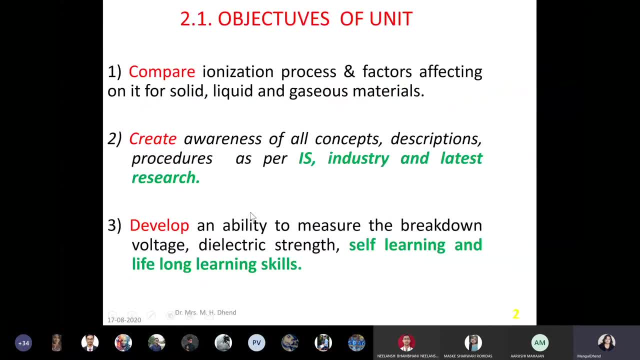 gases, insulating material. so let us start what can be objectives of unit. you must able to compare. comparison is higher level learning. if i will say you describe x, then directly whatever is you have read, whatever i had told, immediately, directly you can start writing. but when comparison is, 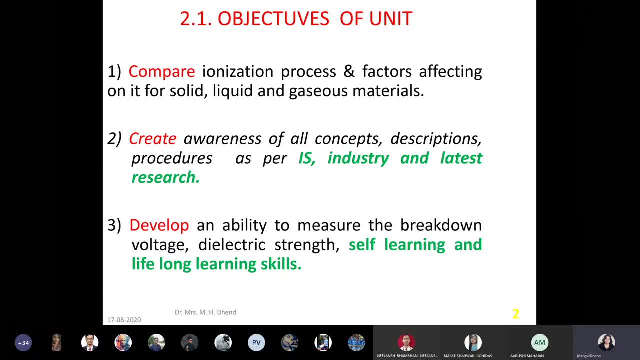 there you have to put your thought in that you have to just see what is the difference, you have to understand, and then you have to apply that while writing. so comparison is higher level, and just now you have gone through the comparison, so that way, here also, you should able to compare. 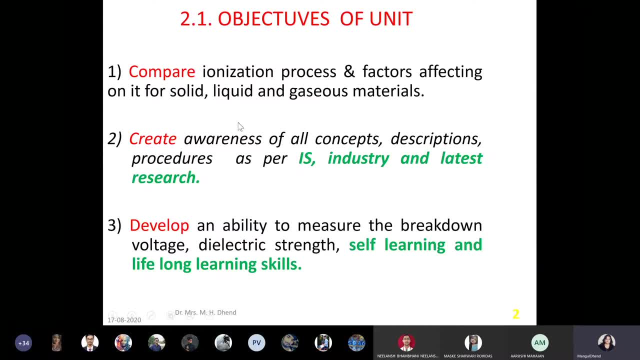 between different ionization process and factors affecting on solid liquid gaseous materials. then create- you should have creations, awareness of industrial procedures, what is latest research is going on. that is also my objectives, or our objective, and you have to show me the outcome. then, third, you should able to develop your 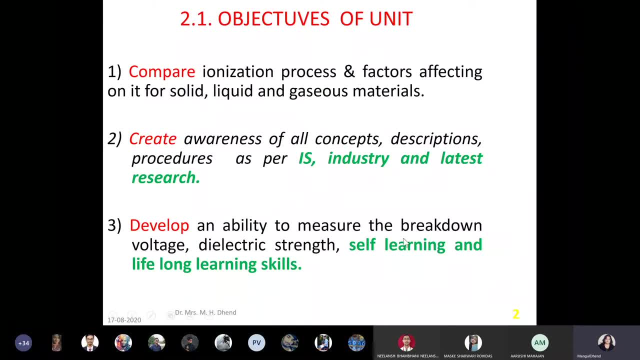 abilities for measuring the breakdown voltage. now, physical lab is not available to us right now, but you can develop your ability to use virtual lab to measure the breakdown voltage of different air gas liquid. so that way we will see in practical. you should able to develop your abilities. 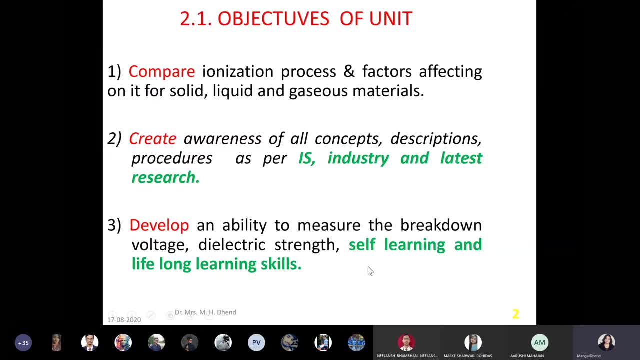 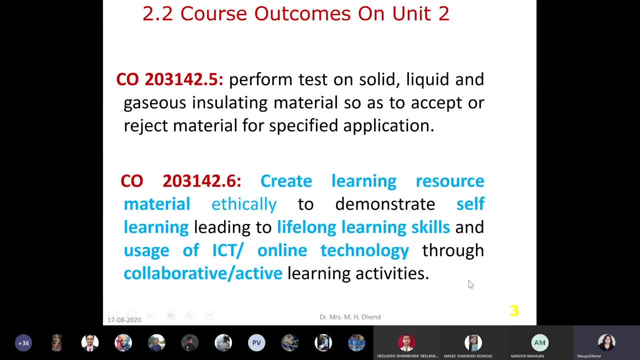 for self learning and lifelong learning skills. many students have already learned themselves virtual lab, oil testing and this. so that way, now, whatever you have learned yourself, that will go lifelong with you. so that is the subject, is what i had kept it before starting this unit. now, course outcome is what you will show as a coupled outcome, so outcome will be if you will attend this. 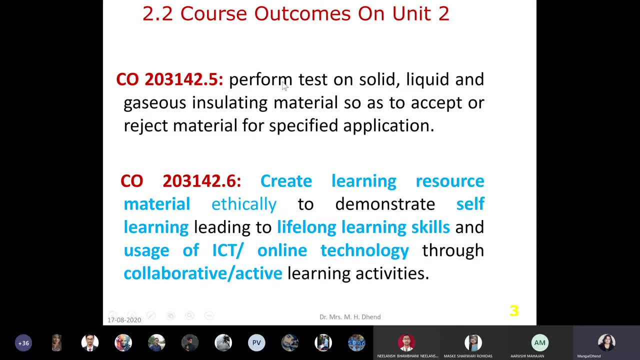 lecture very carefully and attend practical session. then you will be able to perform test yourself. you will be able to perform tests on solid liquid gaseous and also to accept the material or reject the material, because ultimate objective of testing will be: suppose you are testing oil, transform oil, you know now, and you go in market and you ask them: give one liter of. 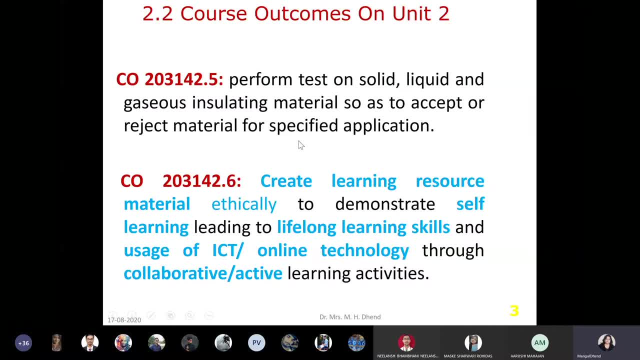 transform oil and now you will learn how to test it. first, you understood characteristics of transform oil. now you will learn how to test it, and you have tested. so whether you will accept the transform oil or reject it, that you will learn here so that your capability should be developed. that will be. 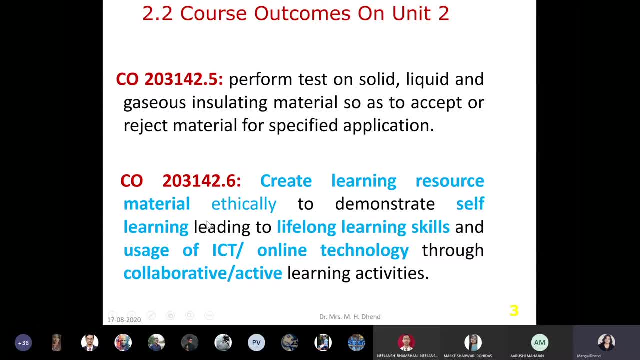 outcome, then you will create learning resource materials ethically. ethically means without copying from other students yourself. you will do, honestly. you will do. you will demonstrate your self-learning skills, lifelong learning skills. already you have done it, but see the u-sales of ICT and online technology, because I had given you that you can take any unit of 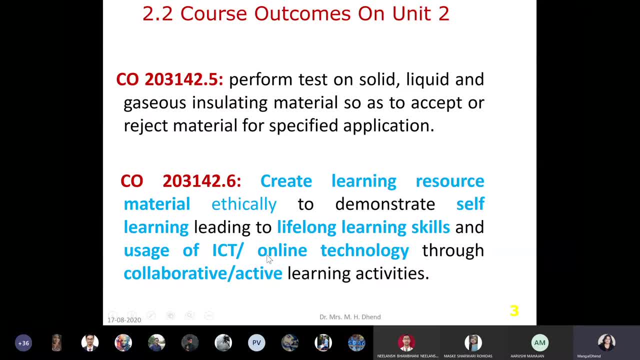 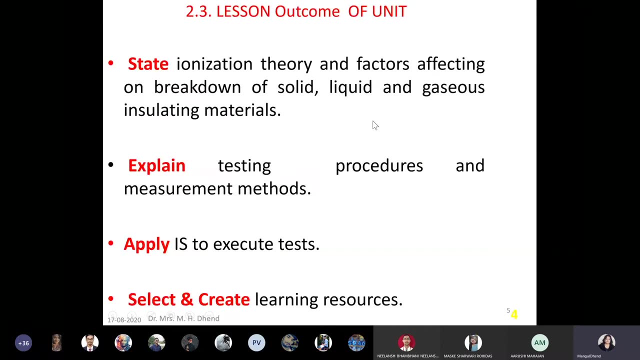 choice in content of your choice and use ict tool available and apply that to any topic. that this part. i think i am very satisfied with your activities. so already this was objective, so you have taken this. only few students are remaining, so that we will see. so you should also will able to state. 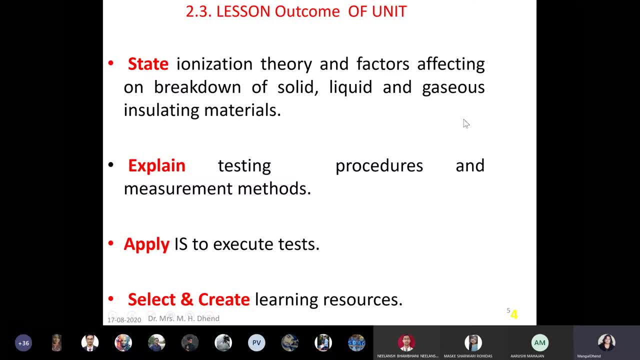 ionization theory. what are the factors affecting on the insulating materials of liquid gases, solid? you will also able to extend testing procedures, measurement methods. you will able to up hundreds to execute tests. so i will give you one is. i will scan it. i have taken from college. 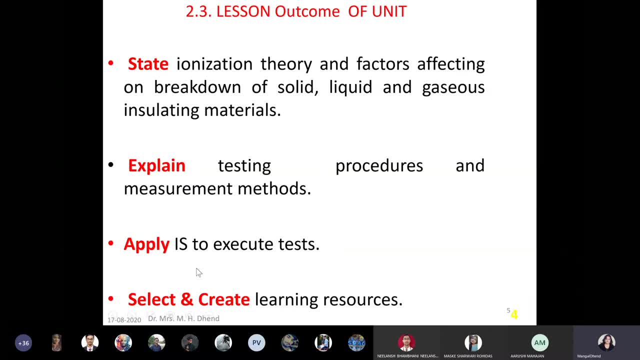 just in last week i had gone, i took the copy, i will scan it and i will give you okay. so that way you go through eyes, you will come to know what is mean bias, and by reading eyes you should able to execute any test, because when you will join the industry there i will not be there. how to taste it. 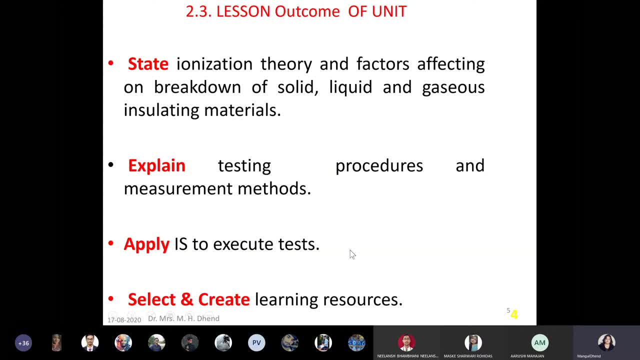 and nobody will be there and you can open internet and you will test number of wrong things can go. because whenever you test, safety precaution has to be there, cleaning precaution has to be there and some standards- international standards, indian standards- you need to apply. so you must know that. 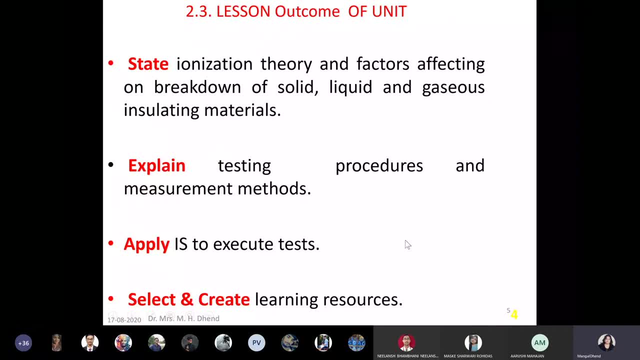 way and what is is so go through. that is. that is also one activity in practical b. you select, that will select that to them i will give to have some abstract on that indian standard. so again, now that date is approaching 20th august, you complete your google sheet leaders, you monitor. today i will call. 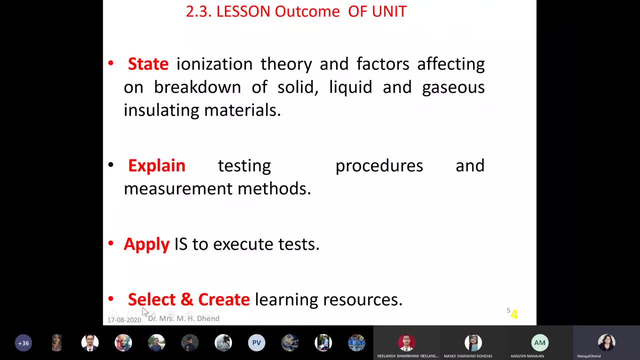 you in the evening and i will check how many of you have completed activity sheet, which you will complete that way. you have to plan it. so what activity is their indian standard and you will be able to apply to execute any test. i will also tell you my case story when i joined the college. 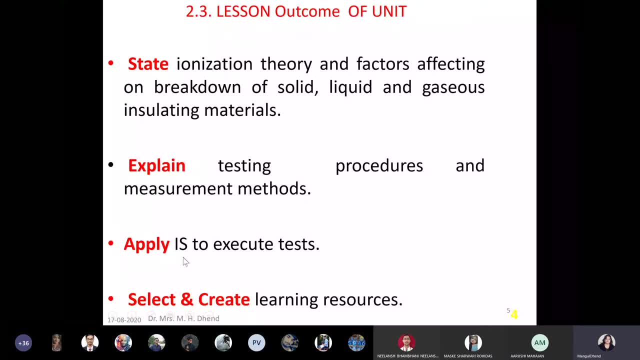 and what happened and how i took help of indian standard to complete my task to accept or reject our device in the lab. that i will tell you. so that way it's very important. you must learn how you can do the task yourself, select and create learning resources. so definitely you have started doing. 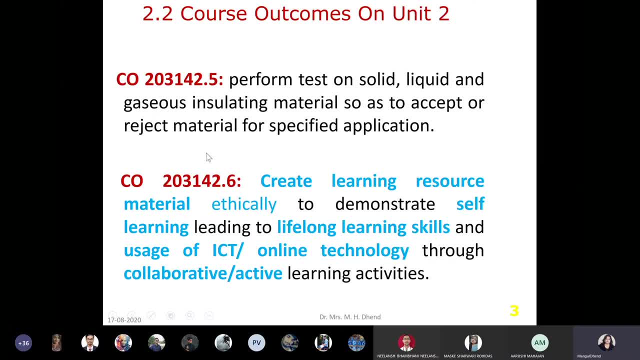 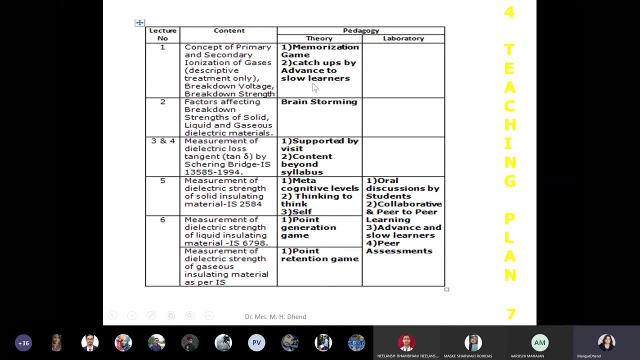 that one activity. you can say it is completed. you created very good learning resources, so that way you can see. on unit two, i had set up objectives and you will show me the outcomes. uh, now, what can be pedagogy? now you come to know i use different pedagogy while taking the units. now, for this unit, pedagogy will 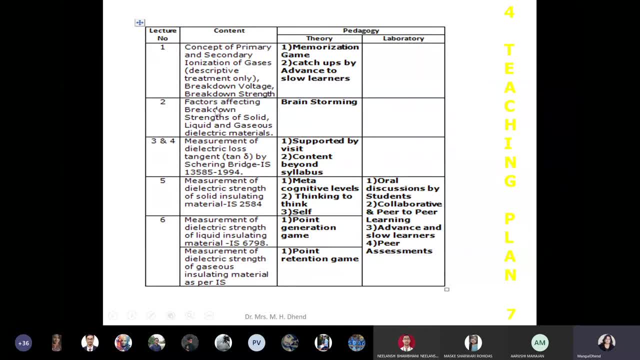 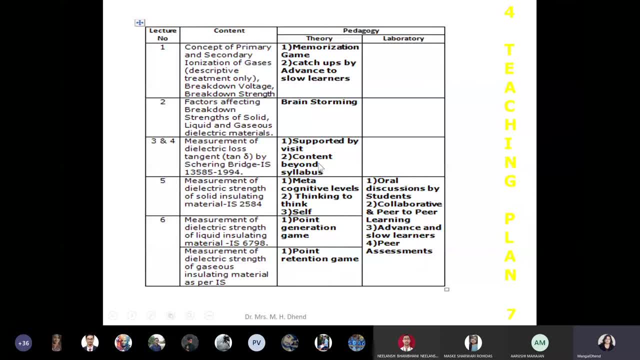 clear the concept and for measurement visit i had planned- now this plan is before missing vacation, but still covid situation continued. so let us see how we can replace this visit for this, where i wanted to take you in madhav capacitor and show you actual this shearing. 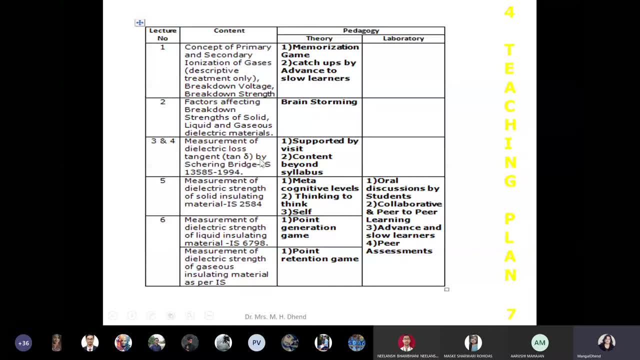 bridge there, but we will wait and we will replace this. i will tell you what i have thought just now for this. i will take competition now. this unit will be full of competition, and what kind of competition will be there? i will get everybody's response with your name, only first top 20 students. 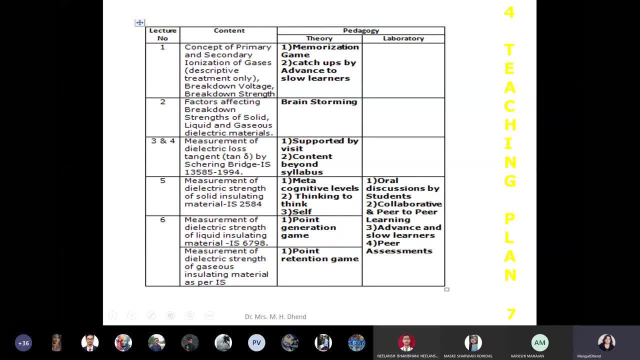 because they accept only 20 fast responses and depending upon your time of response you will get mark. suppose i have responded within one minute and you have responded within 1.1. then you will get less marks. i will get higher marks so that we will see who are very sharp students in the class and who respond very fast and whose. 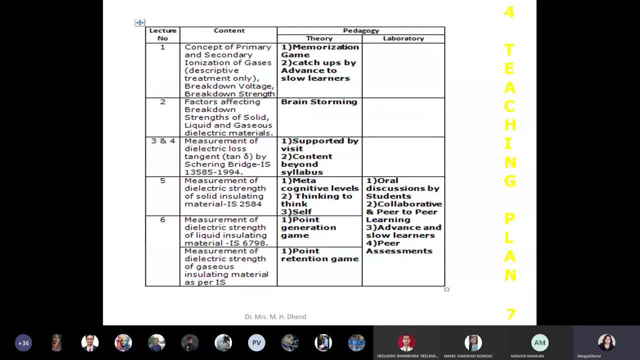 score is what, and you will immediately come to know your answers are correct and wrong, and also we will able to declare our first winner in the class. not only first winner. all 20 will be ranked in the sequence. so that way, just be ready yourself a lot of competitions. i will start in this unit. 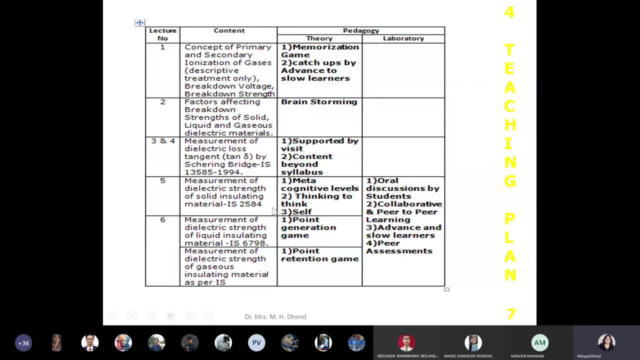 then measurement of dielectric strength of solid liquid insulating material. we will also focus on metacognitive levels, means like you will think, and you will think to think, learn to or think to think, think how to think. so that way we will see. now you know the memory map. 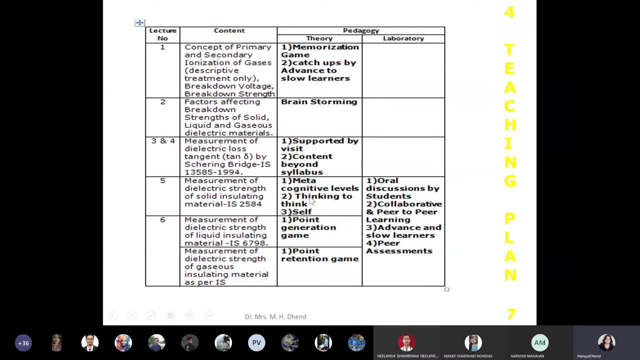 concept. so here we will just focus in the depth and then point generation game, you know it, point retention game we will play now. okay, in this unit you will create a memory map and one memory map will take and all students will focus on that memory map to return the points and let us see who can. 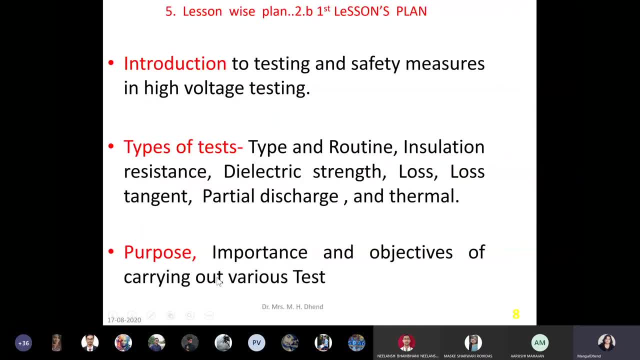 return maximum points that games will play. so be ready yourself to have active participation. don't just log in. i will come to know now who has only login and then lesson wise plan. i have made now lesson wise plan, first introduction and then testing. a brief. i will tell you okay, and then i 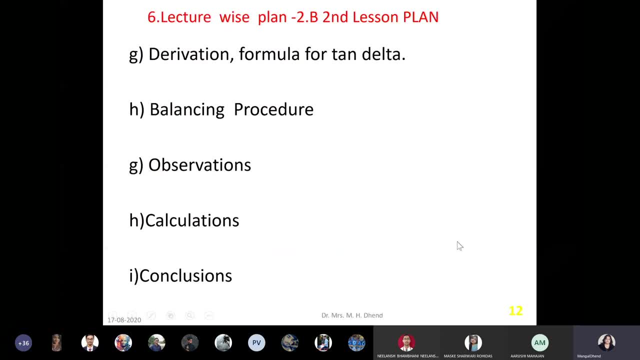 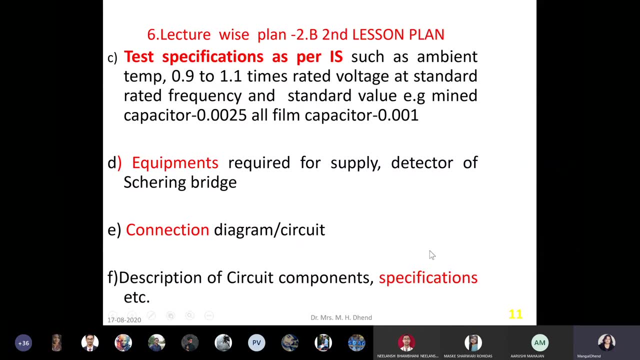 will go also. i will tell you in next lecture. now first, before starting, i will like to tell you whatever test we will discuss it. you should able to write down the test with equipments, which equipments we use, what should be connection, how to draw circuit diagram, what are the specifications. 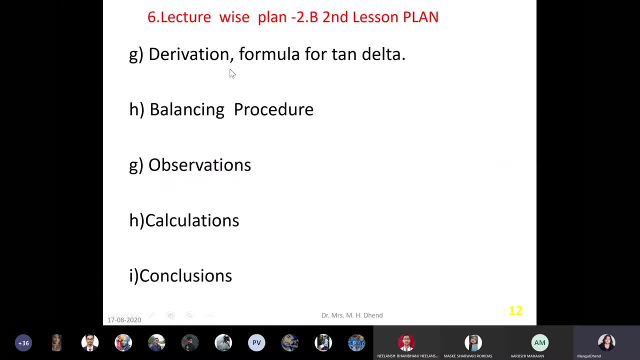 of each device. derivation of formula: if is required, what formula? that is only for 10 delta, okay, then balancing procedure: if procedure we have to follow, then observations, calculations, conclusions. now you know all this because you have performed experience in first year. so what else new is here? 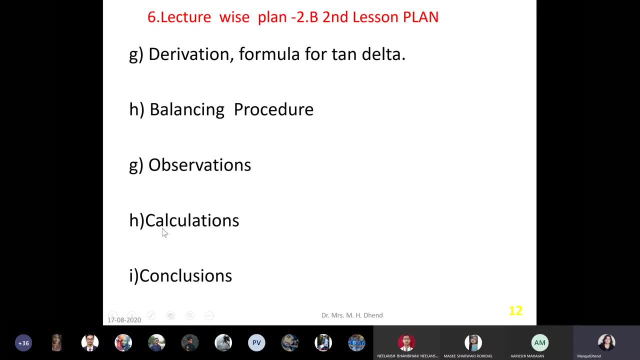 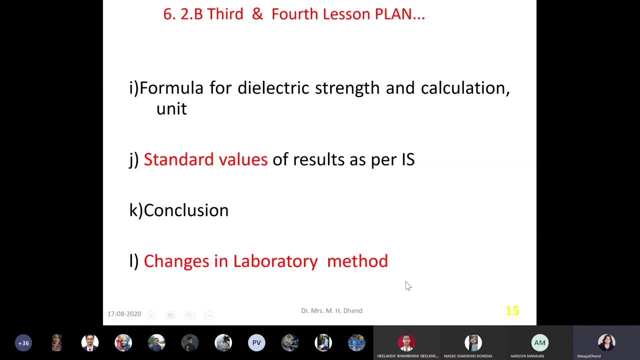 new is nothing, but under this point you must able to write down. so, even if it is theory, you have to write down. this way only, and that way only you start attending lectures, what you can write down, that. so that is what i want to tell you, to tell you my objectives now, what will be teaching activities? so just now, we will start with my one. 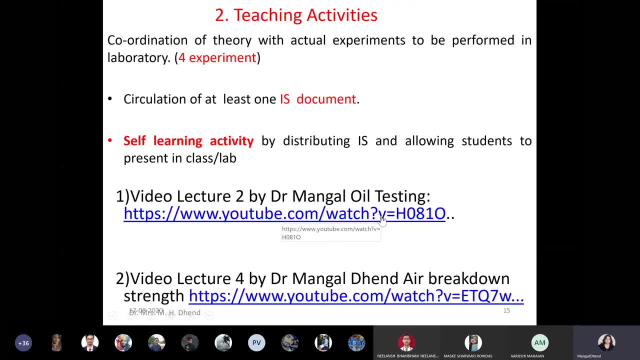 video of oil testing, because i am starting with first test measurement of dielectric strength of oil, how we can measure dielectric strength of oil, how we can measure breakdown voltage of oil. so for first, watch the video and then we will discuss. keep your notebook ready, have some. 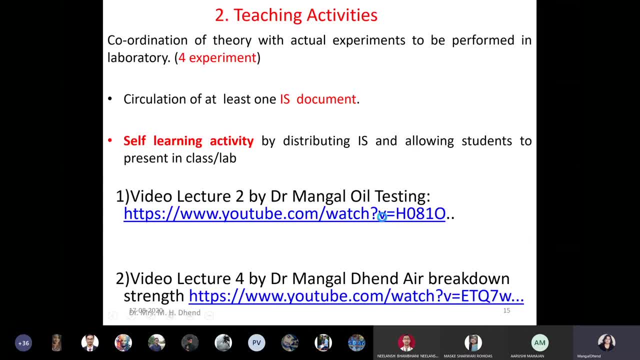 points and then we will discuss how to measure dielectric strength of oil. so first watch the video, Stop the video, and then how to measure dielectric strength of oil. are you ready? now, just look, you need to have that tape of some machines. what do we do? 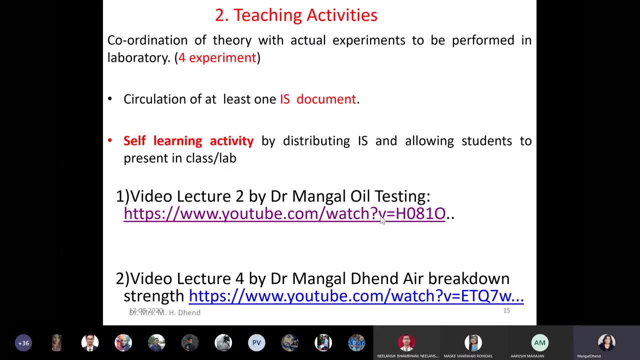 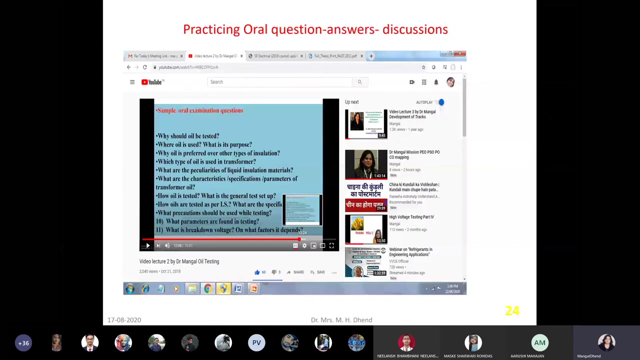 okay, what can you achieve? um, uh, available, I don't know. okay, my video is not. can watch. I will post a link in our group. you watch the video before we start discussing that experiment. okay, so in video I have discussed number of questions because when we see this as a 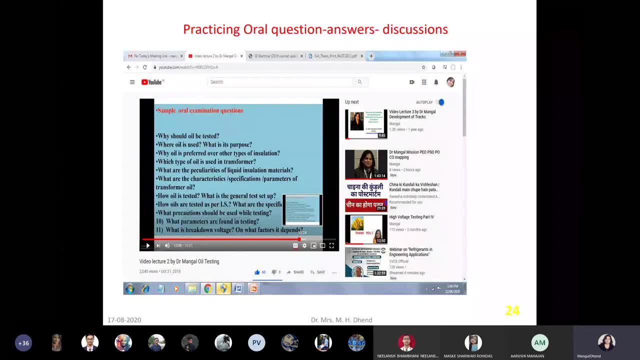 theory part. you must able to write down the answers with the points like objective of the test, then apparatus specifications, safety precautions, equipment, procedure, calculations, observation table, conclusion, like that. that you know. but when experiment you will perform virtually- now I will say virtually- oral exam will be there, you identify, marks are there for oral and 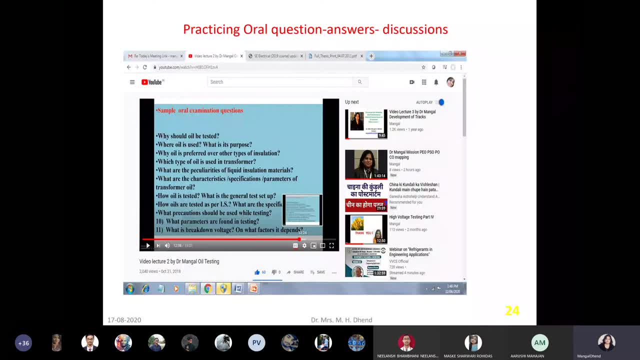 This year it's new to you because second year students are not habitual with oral exam. So on oral exam, what type of questions will be asked on the same experiment that I have discussed in video. So you attend, you watch video and then we will discuss in our lecture how to perform that experiment, and theoretical aspects I will discuss in the lecture. 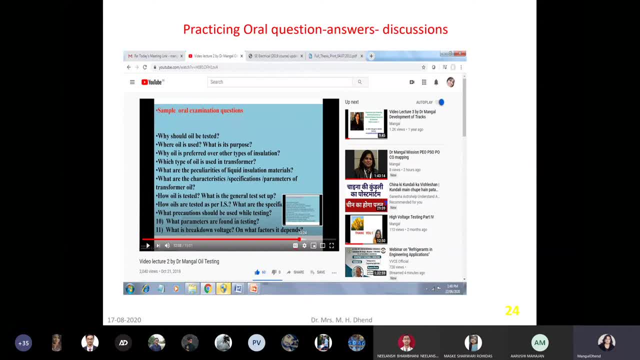 And the same oil testing experiment we will take now in this week, practical, And in the practical we will watch virtually how your classmate has done that, used virtual lab And side by side you will perform that experiment virtually. You will have your own reading. 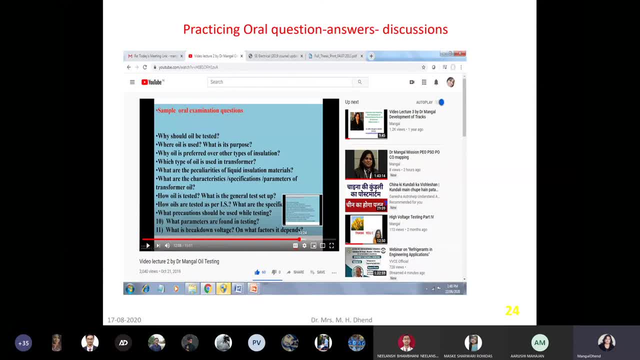 You will write down in your notebook and from your own reading you have to plot graph and write down conclusion And then we will discuss oral questions In the practical. So that way it is a plan means hand in hand, theory, practical, theory, practical. 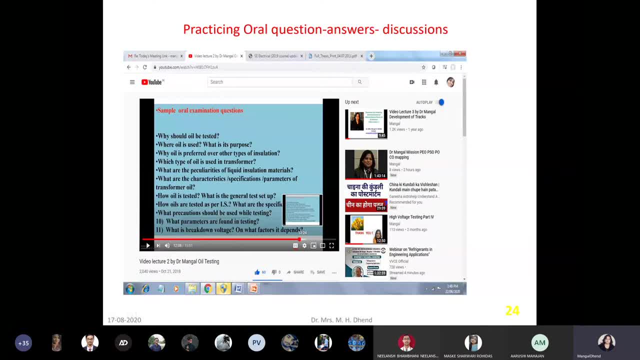 So that way I think it will beautifully clear you all concepts and better understanding of theory, and oral exam also will be done. So today you watch this video. It's just meant for the exam And I will share my experience with this video when I launch it two years back. 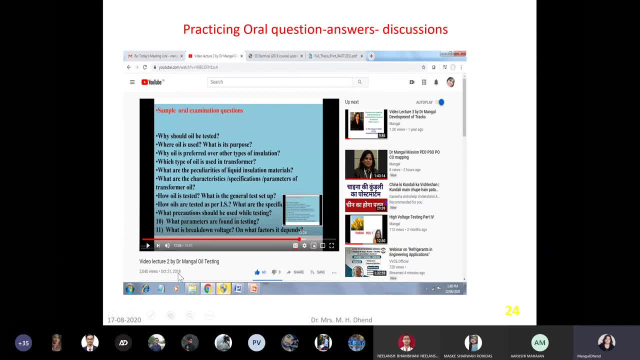 See the time date: October 2018. after the video went in other colleges and all examiners said me, madam, that you are videos to experiment students answers so nicely and really performance was very good because all the oral questions students could understand it as discussed in the video. 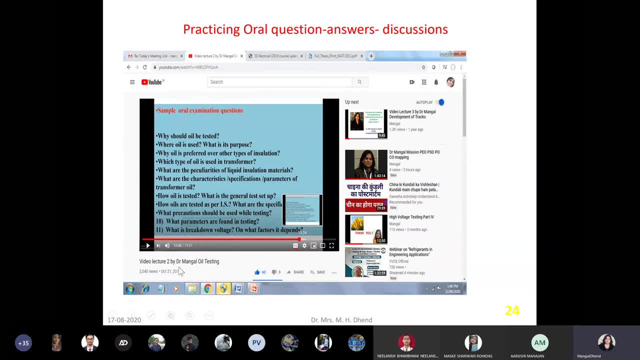 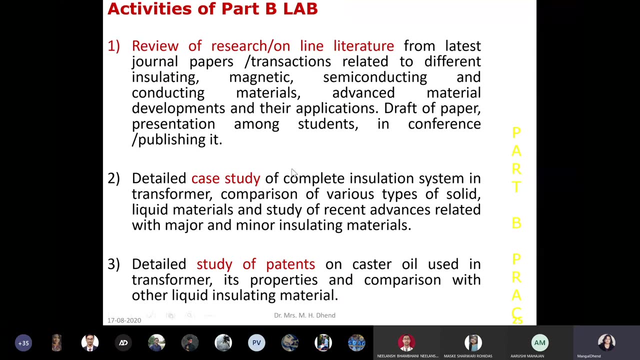 So that was the feedback which I had received for this experiment to three experience which launched in Two years back. so that way I am now telling you you watch for send, Then we'll discuss again. more strong impact will be there. Okay, so that is what one is. their activities are there. now you can start research paper activity. 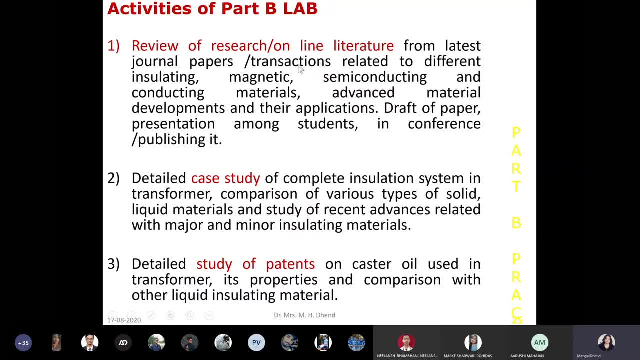 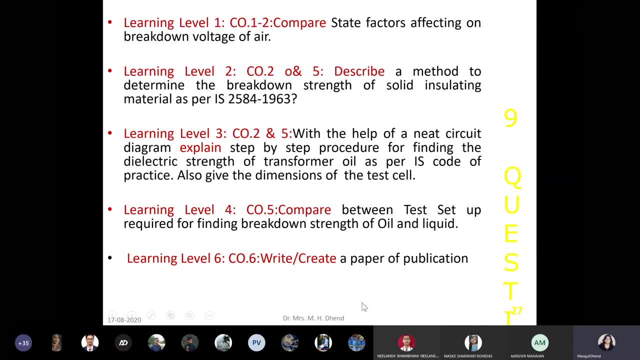 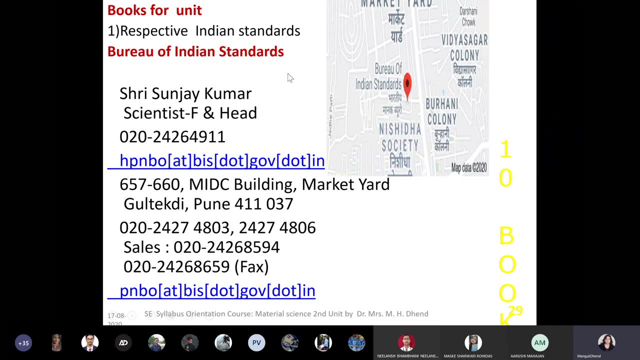 I will take one lecture, how to write down paper, and then you can write down research paper related to this unit, case studies, and so their patent is also there already. I have told you. so now books for this, This unit. so book for this unit. if you see, measurement part, ISE is required. so ISE is having copyright, so I cannot post to you. but whatever it mention is in ISE that I have written in my book in simple way. 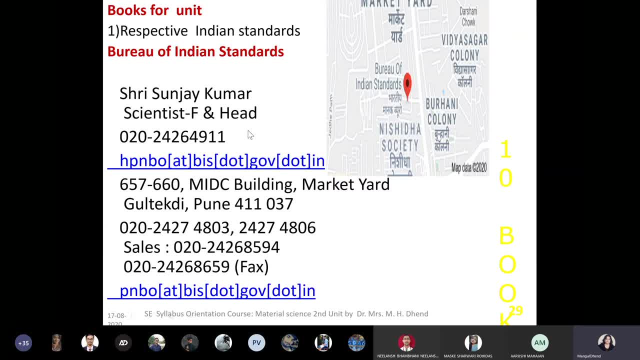 I'm reading copyright issues, so that way I am posting you my book or scan copy. I don't know whether you have referred for the test. you refer it. What A problem you paste with that you tell me, because scanning some matter might have cut so that. 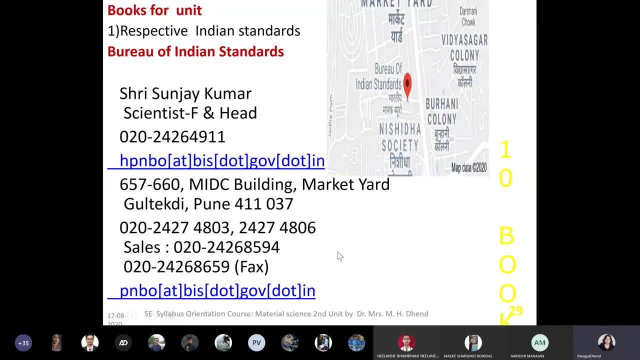 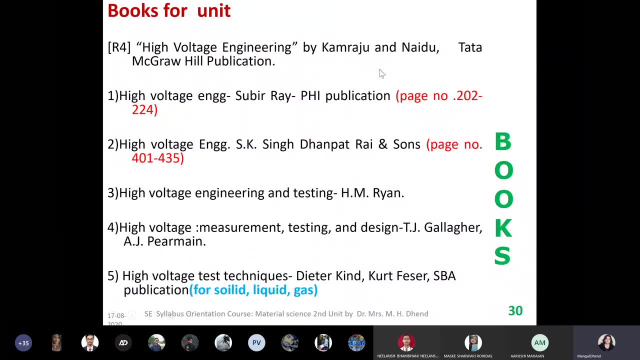 We will learn when I as, but I as directly, I cannot give you all the eyes, okay, so that is one thing. now, book you had to write down. write down the book Again and again. you should not ask me because I am giving you unit wise, no book, because only one book will not sufficient. so 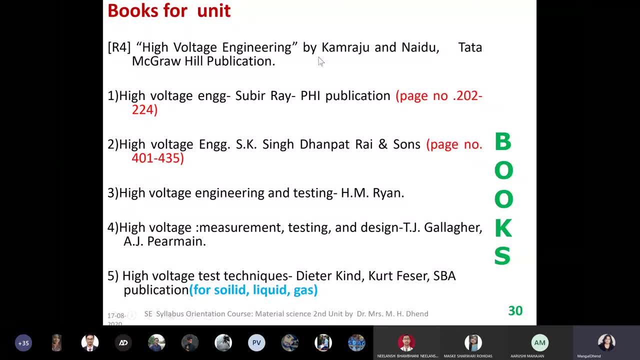 For this you you must refer High Voltage Engineering by Kamrojanadu that you ask me scan copies of this book for the unit content of this. I will mail you, post you, okay, but you write down: you have to refer this book, not material science book. this is High Voltage B book. you have to use it because in 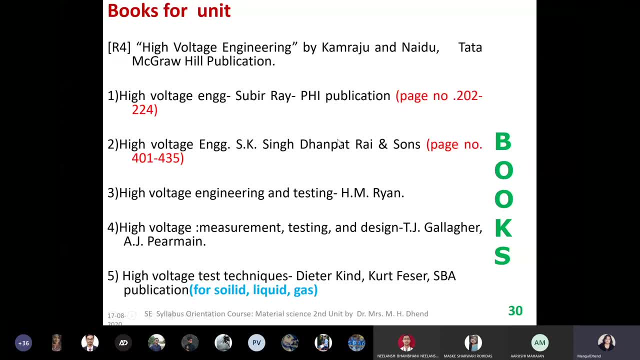 material science book. this part is not there and other: this book will be required for oral, but already I have discussed in my videos. so this book. even if now you don't refer library that way is your problem, okay, but I have already referred this in our video. so now let us start. 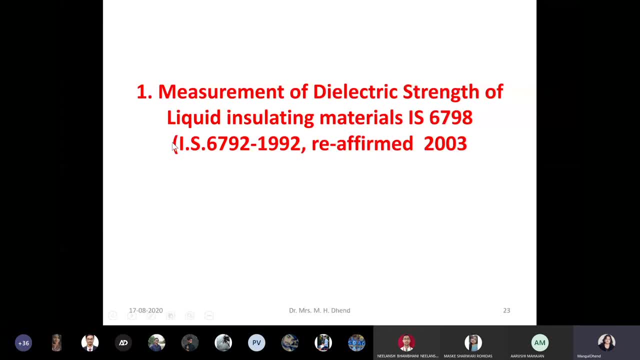 with first experiment. write down our first measurement method out of four is measurement of dielectric strength of liquid insulating material. IS number you have to remember: ISC 6798 1992. so this is the Indian standard number is given. it was established in 1992 and reaffirmed. 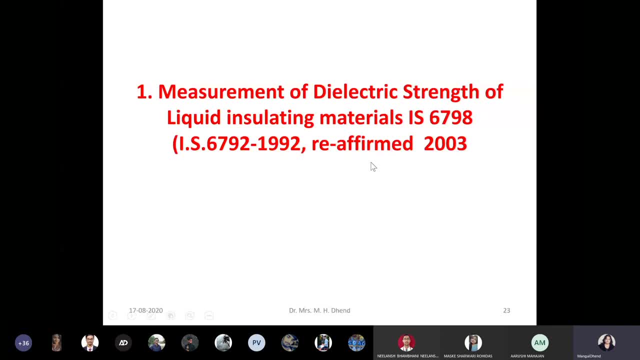 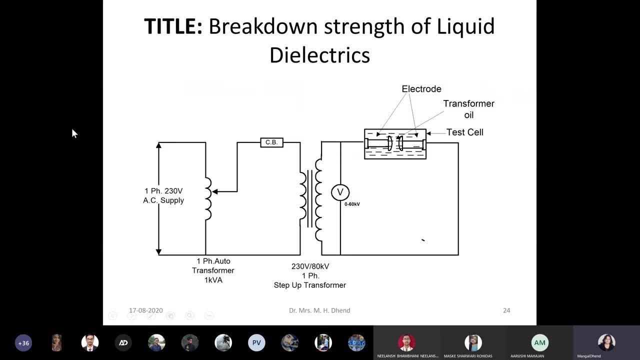 in 2003 means after so many years, again people went whether the content of this Indian standard is good. weather changes are there, so it is reconfirmed in 2003 and still India is using this standard. okay, so test circuit diagram: is this now already? I have explained, you suppose, here oil we have taken to find out breakdown. 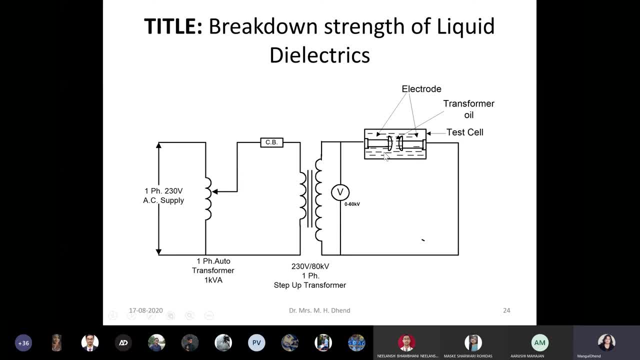 voltage or dielectric strength I already discussed in my first week lectures. so now you want to find out breakdown voltage of liquid means. what number of experiments are there on finding breakdown voltage? so you know. now insulating material: you know transform oil is the insulating material and 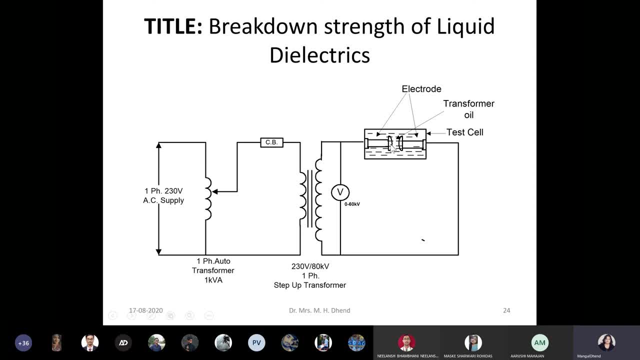 when you will place between the two roads. it should not allow current to flow. so here very high voltage is given, see 60 kilo volt, 80 kilo volt. kilo holes are given, still no current should flow through the oil, because oil is insulating. 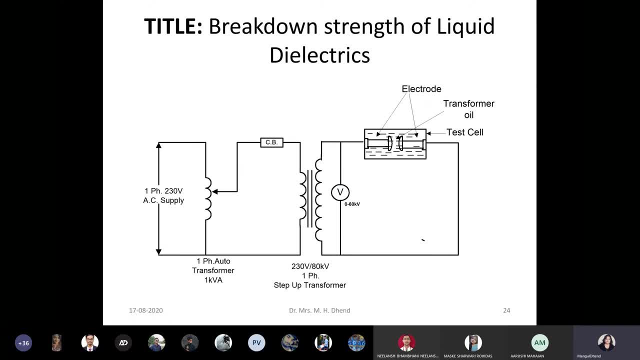 material. okay, but when we are testing measuring breakdown voltage, we will go on increasing this transformer voltage. 100 kilo volt, 80 kilo volt. we have 10 kilo. hole 20 kilo, hole 30 kilo. just just go on increasing voltage and find out at what voltage insulating material will break down. so it 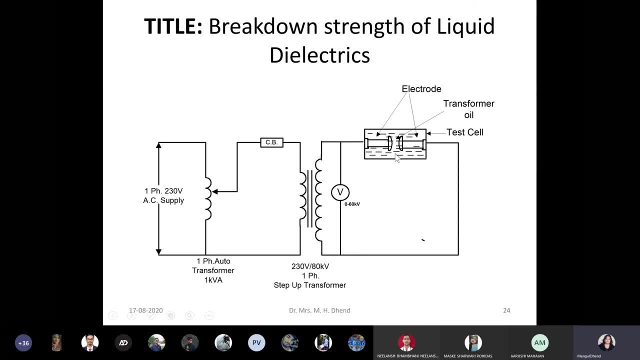 is not physical breakdown, it is breaking down of the insulating properties. already I have explained you. it is the destruction of insulating properties. so at what voltage this insulating material will start conducting- that voltage you had to note- and how you will come to know that um oil has started. 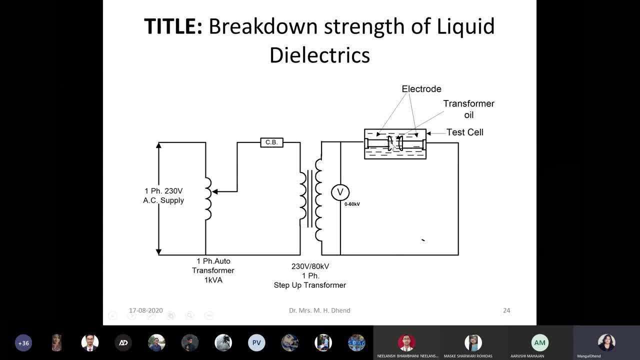 immediately spark will take place because insulating material has start conducting means. now here is no resistance between the two electrode. so what will be resistance in the circuit? only resistance of the transformer, winding resistance of the electrode which is conducting material. and this resistance of oil has dropped down, so dangerous short circuit will take place with a. 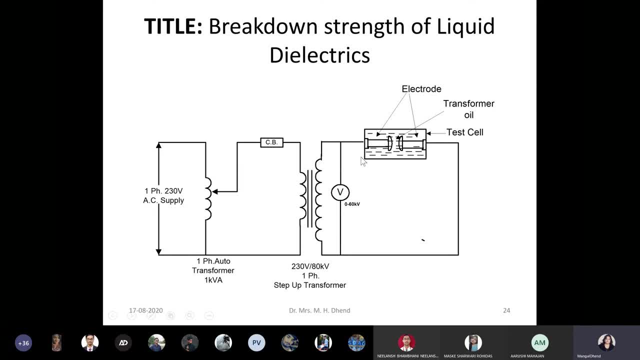 kilo hole. so whole college transformer will go up, wiring will go up and danger, hazardous thing will happen. so immediately here circuit breaker connecting in primary winding will cut off the voltage and spark will take place because that oil will flash over due to the conduction in the oil. so you will observe spark and circuit breaker will trip. so